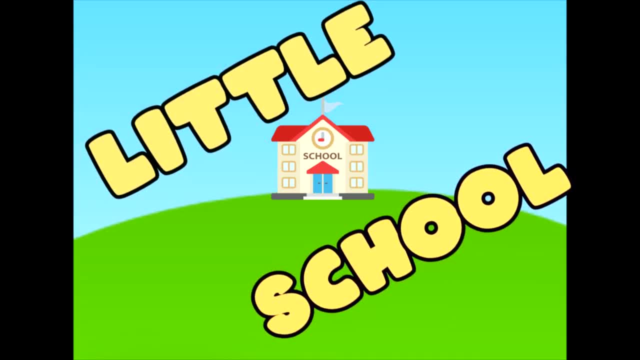 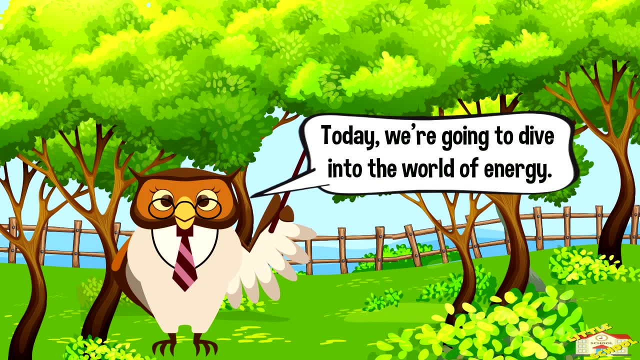 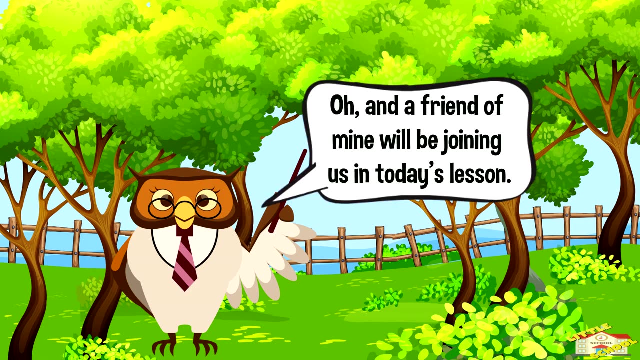 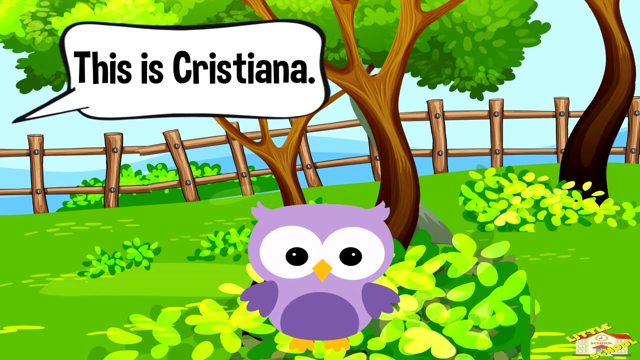 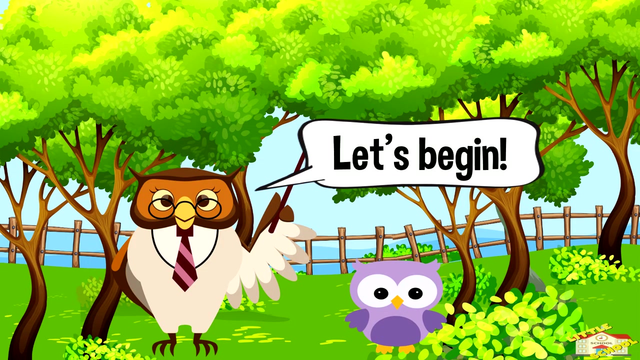 Hey kids, Today we're going to dive into the world of energy, Specifically kinetic energy. Oh, and a friend of mine will be joining us in today's lesson. This is Christiana. Are you all ready? Let's begin. Have you ever ridden a bicycle? 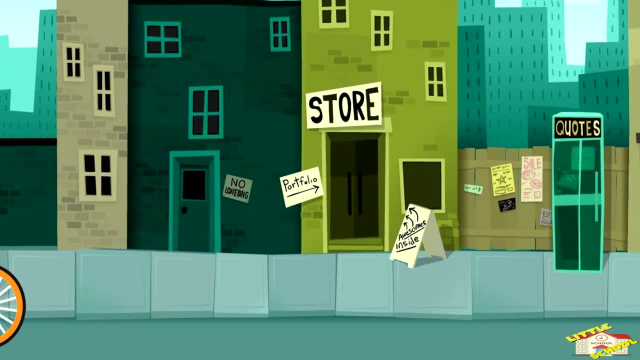 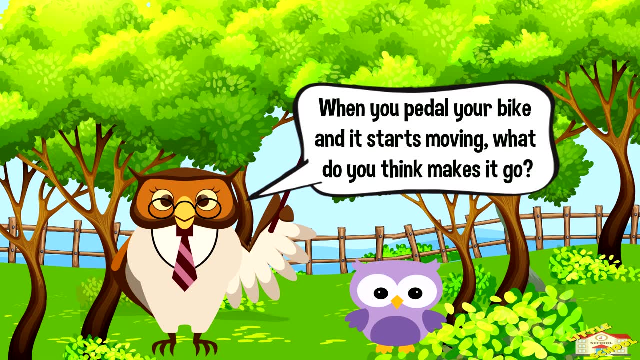 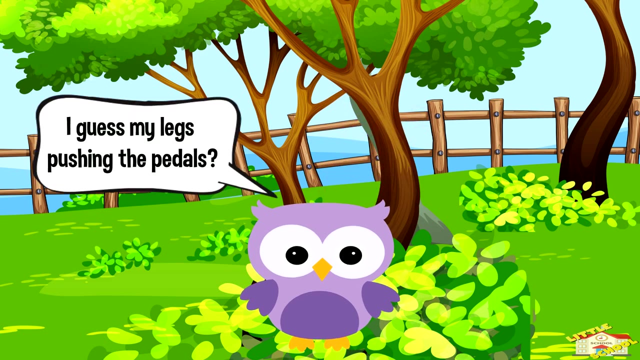 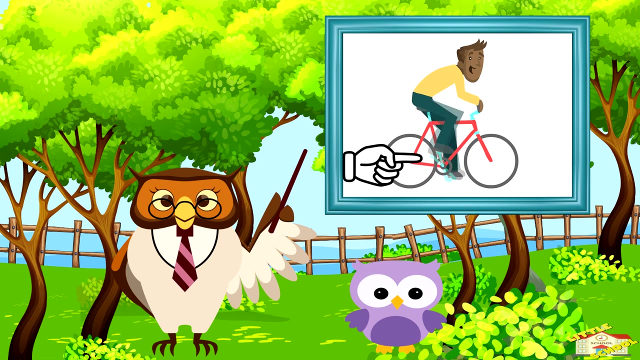 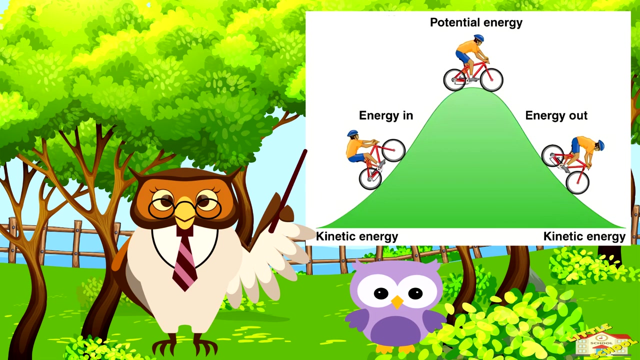 When you pedal your bike and it starts moving, what do you think makes it go? Oh, you got it. When you push the pedals, you're giving the bike energy. And that's where our story about kinetic energy begins. Kinetic energy is the energy an object has because it's in motion. 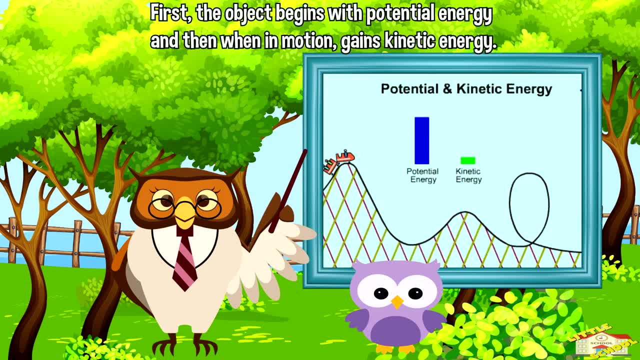 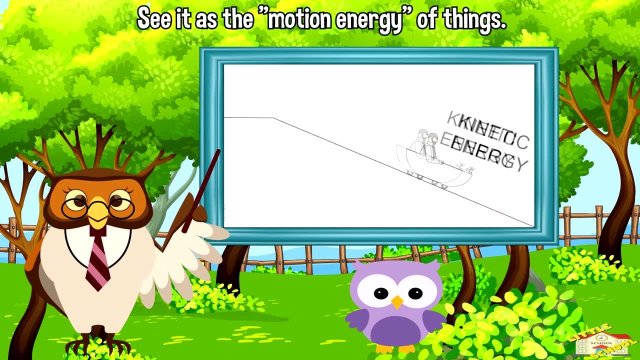 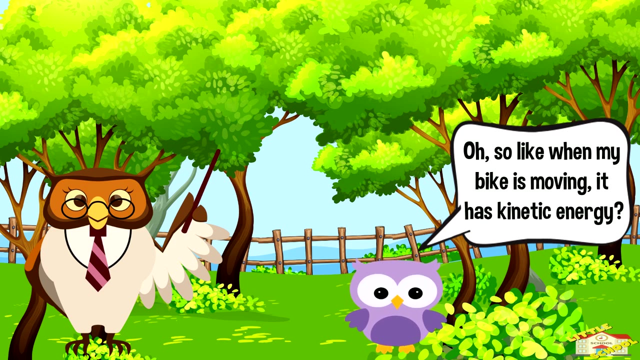 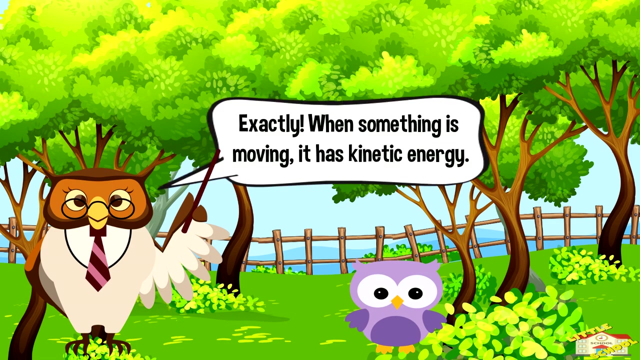 First the object begins with potential energy and then, when in motion, gains kinetic energy. See it as the motion energy of things. Exactly, When something is moving, it has kinetic energy. The faster it moves and the heavier it is, the more kinetic energy it gains. 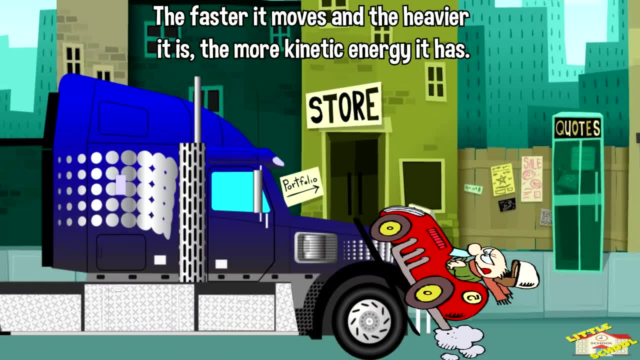 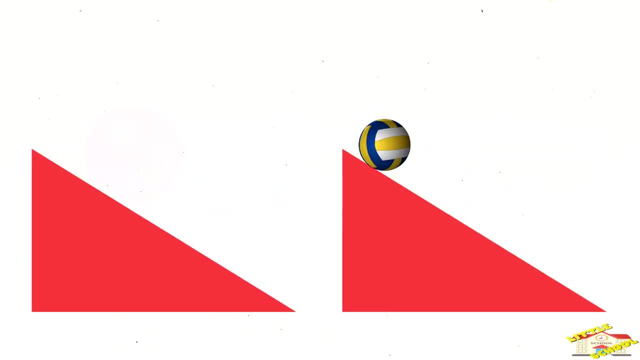 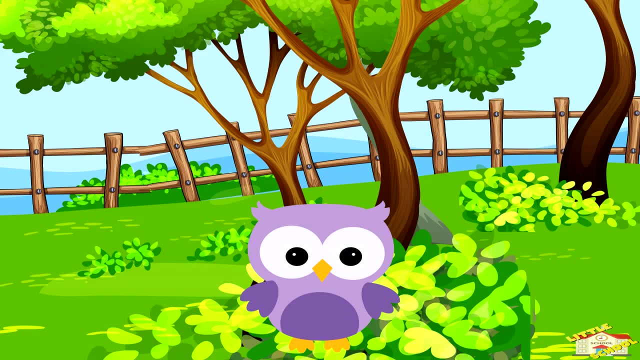 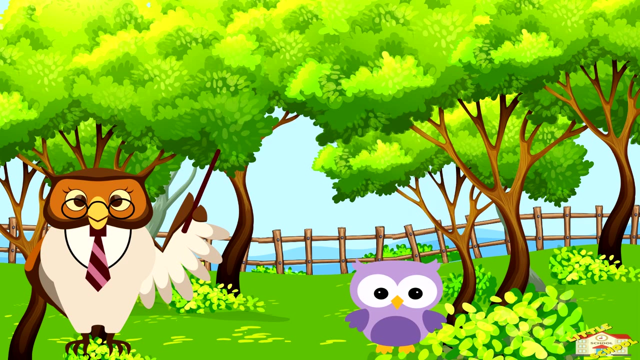 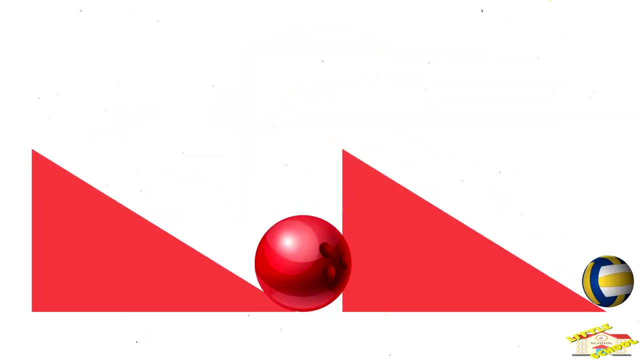 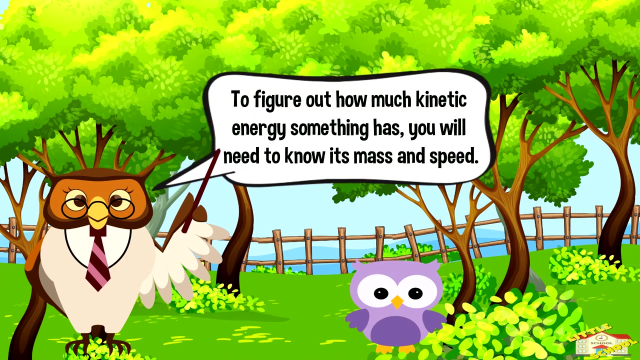 energy it has. let's imagine a ball. if you roll a small ball and a big heavy ball at the same speed, which one do you think has more kinetic energy? you're right, the big heavy ball has more kinetic energy because it has more mass and is moving at the same speed as a small ball. to figure out how much.